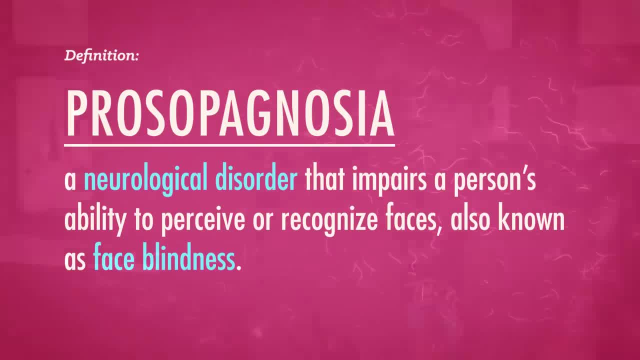 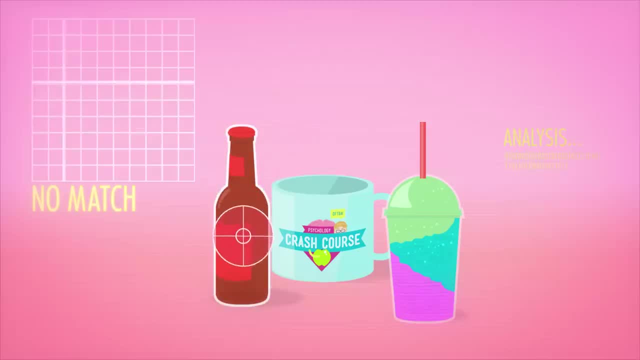 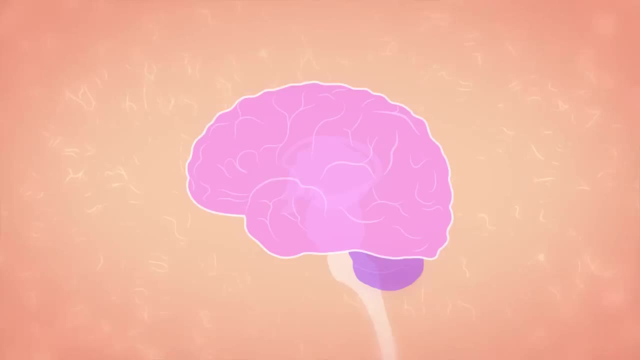 or recognize faces, also known as face blindness. Last week we talked about how brain function is localized, and this is another peculiarly excellent example of that. Sacks can recognize his coffee cup on the shelf, but he can't pick out his oldest friend from a crowd, because the specific sliver of his brain responsible 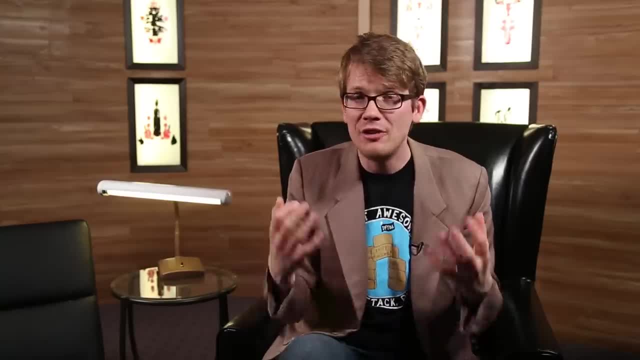 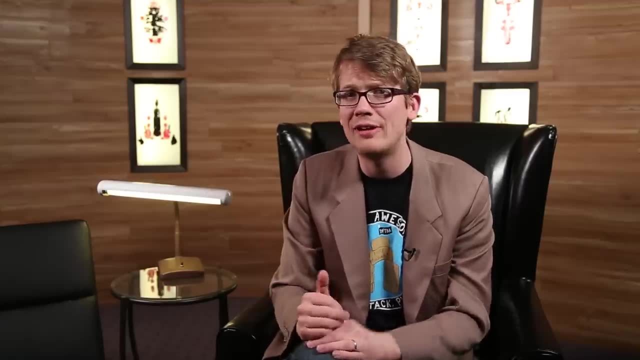 for facial recognition is malfunctioning. There's nothing wrong with his vision. The sense is intact. The problem is with his perception, at least when it comes to recognizing faces. Prostopagnosia is a good example of how sensing and perceiving are connected. 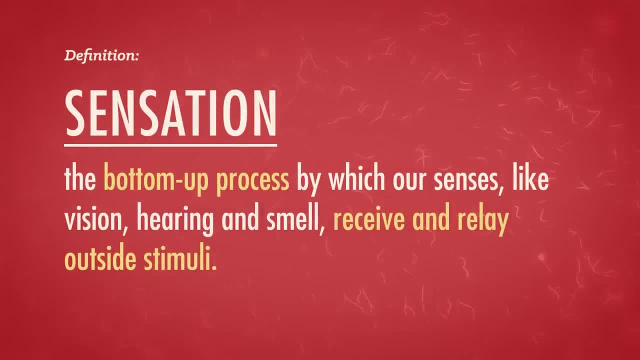 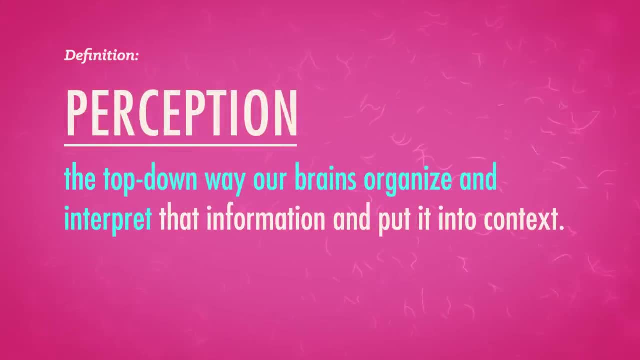 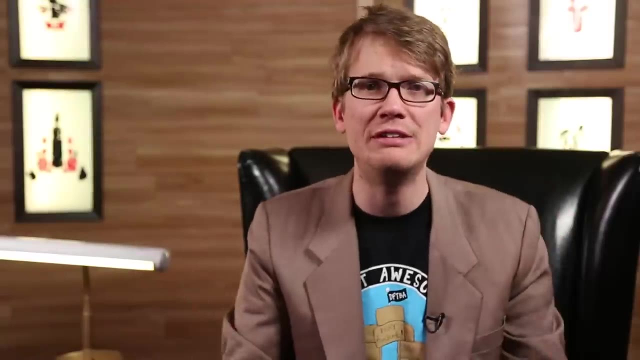 Sensation is the bottom-up process by which our senses, like vision, hearing and smell, receive and relay outside stimuli. Perception, on the other hand, is the top-down way that our brains organize and interpret that information and put it into context. So right now, at this very moment, you're probably receiving light from your screen. 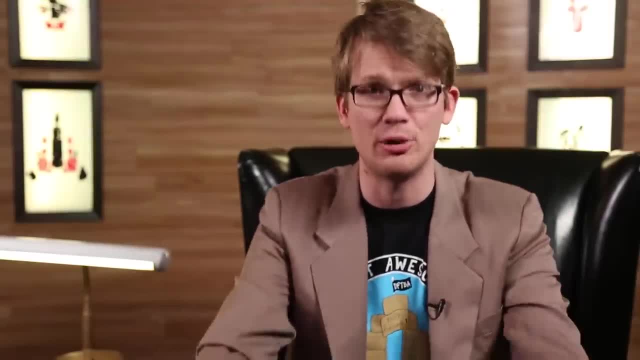 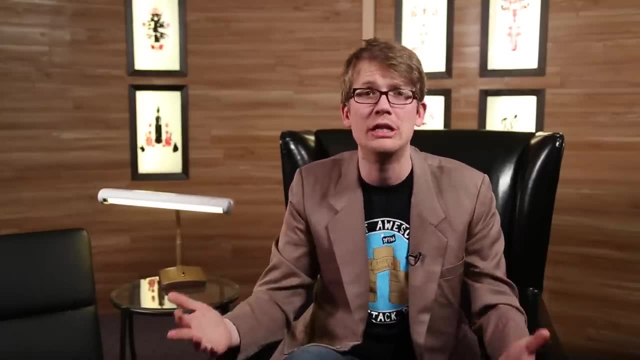 through your eyes, which will send the data of that sensation to your brain. Perception, meanwhile, is your brain telling you that what you're seeing is a diagram explaining the difference between sensation and perception, which is pretty meta. Now your brain is interpreting that light as a talking person whom your brain might. 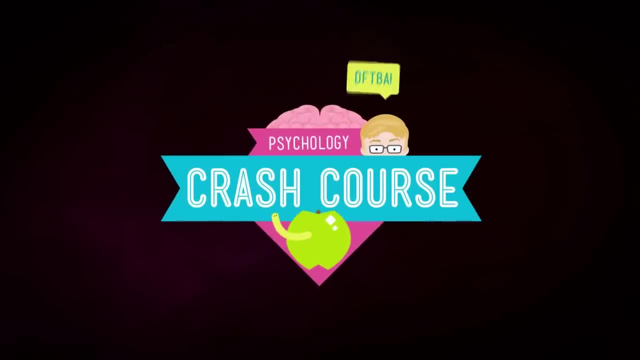 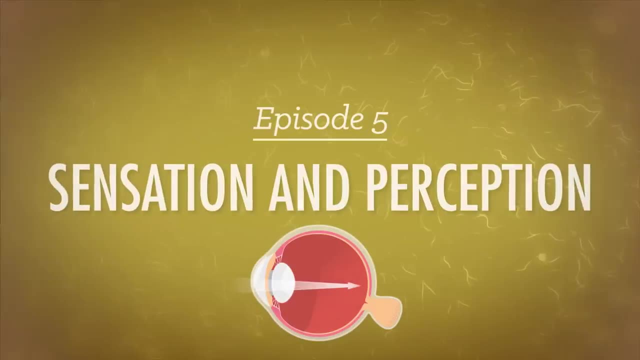 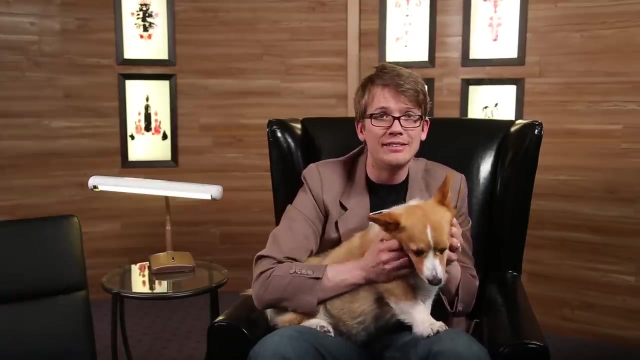 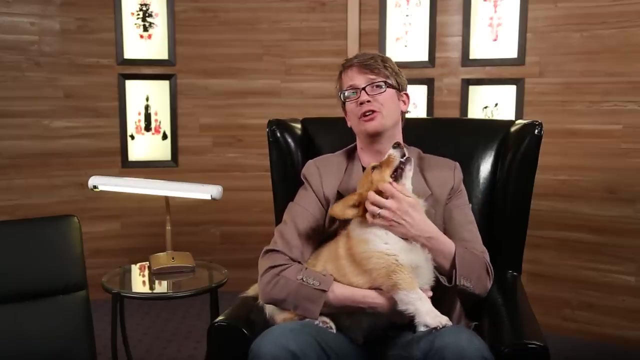 additionally recognize as Hank. We are constantly bombarded by stimuli, even though we're only aware of what our own senses can pick up, Like I can see and hear and feel and even smell this corgi, But I can't hunt using sonar like a bat or hear a mole tunneling underground like an owl. 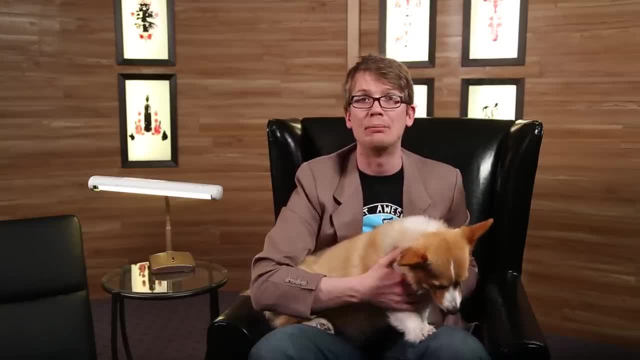 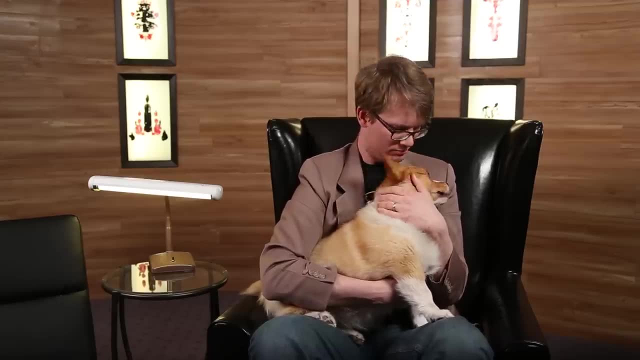 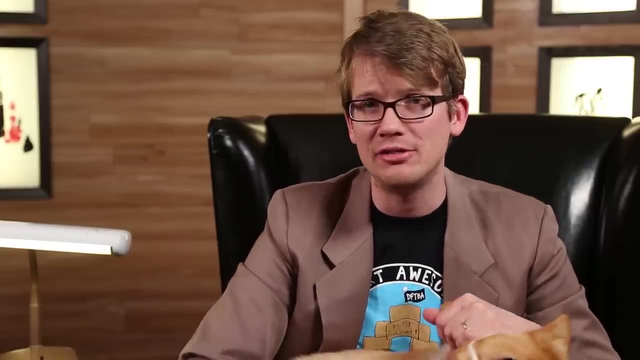 or see ultraviolet and infrared light. like a mantis shrimp, I probably can't even smell half of what you can smell. No, No, We have different senses. Yeah, There's a lot to sense in the world and not everybody needs to sense all the same stuff. 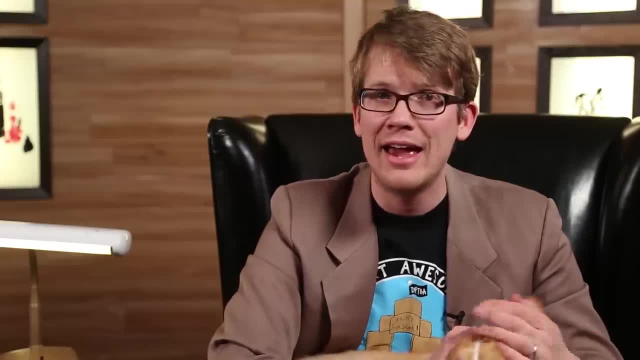 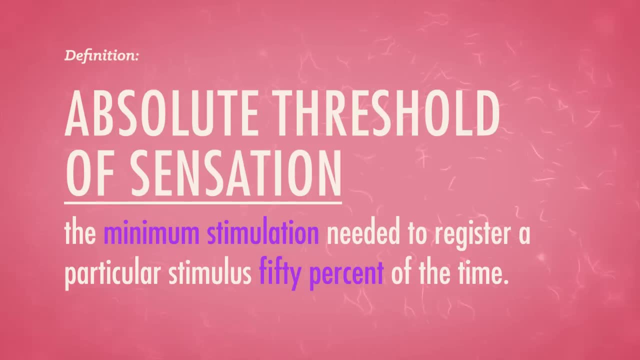 So every animal has its limitations, which we can talk about more precisely if we define the absolute threshold of sensation, the minimum stimulation needed to register a particular stimulus: 50% of the time. So if I play a tiny little beep in your ear and you tell me that you hear it 50% of the times that I play it. 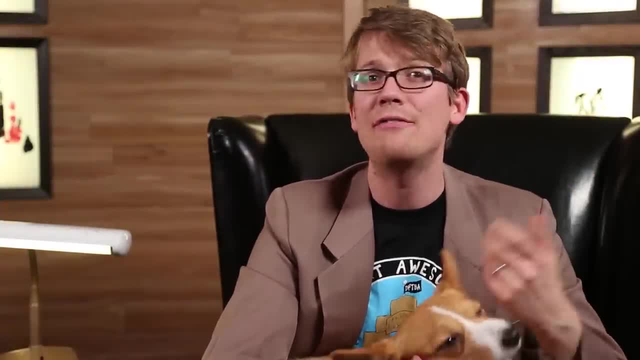 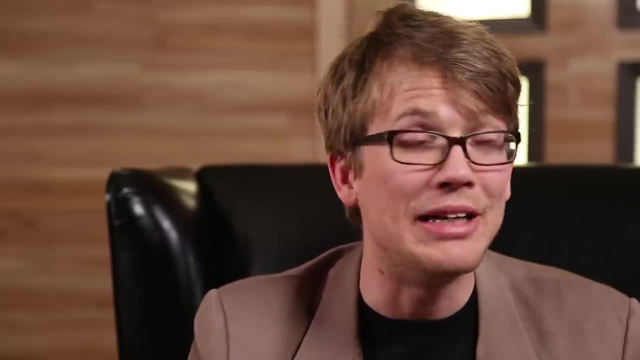 that's your absolute threshold of sensation. We have to use a percentage because sometimes I'll play the beep and you'll hear it and sometimes you won't, even though it's the exact same volume. Why? Because brains are complicated. Detecting a weak sensory signal like that beep in daily life isn't only about the strength of the stimulus. 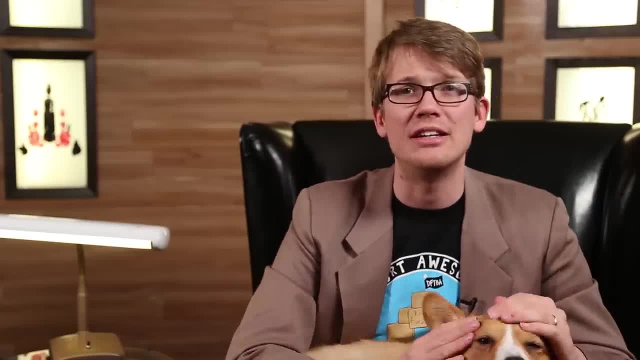 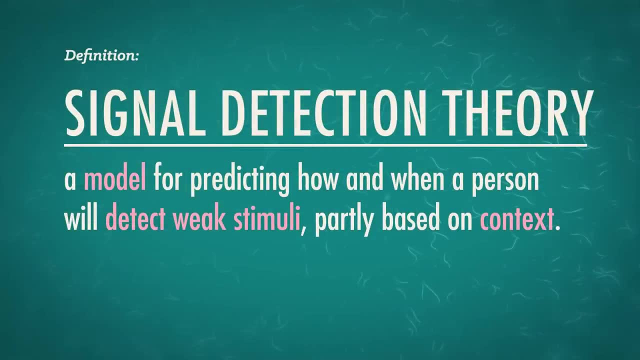 It's also about your psychological state, your alertness and expectations in the moment. This has to do with signal detection theory, a model for prediction, predicting how and when a person will detect a weak stimuli, partly based on context. Exhausted new parents might hear their baby's tiniest whimper. 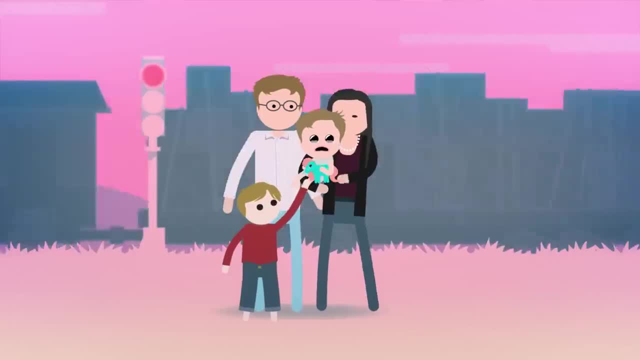 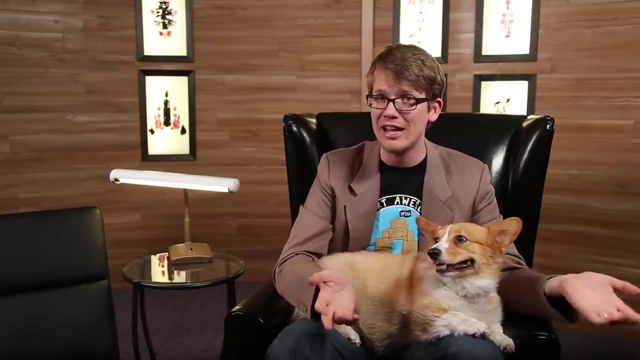 but not even register the bellow of a passing train. Their paranoid parent brains are so trained on their baby. it gives their senses a sort of boosted ability, but only in relation to the subject of their attention. Conversely, if you're experiencing constant stimulation, 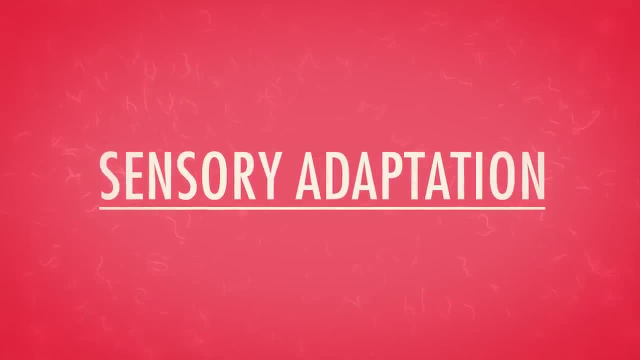 your senses will adjust in a process called sensory adaptation. It's the reason that I have to check and see if my wallet is there, if it's in my right pocket, but if I move it to my left pocket it feels like a big, uncomfortable lump. 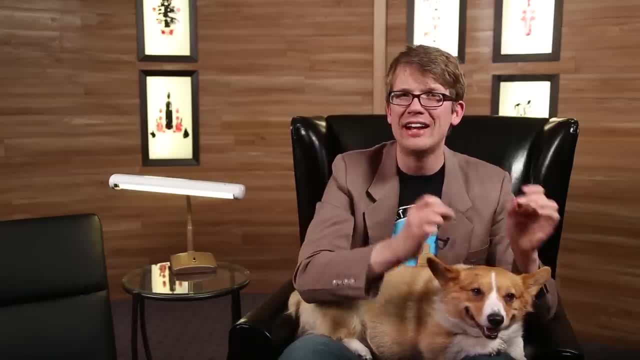 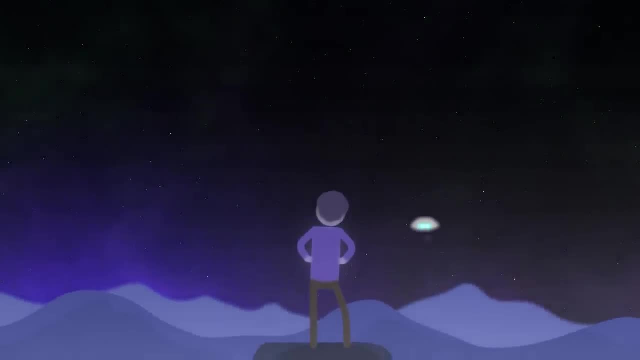 It's also useful to be able to talk about our ability to detect the difference between two stimuli. I might go out at night and look up at the sky and well, I know with my objective science brain that no two stars have the exact same brightness. 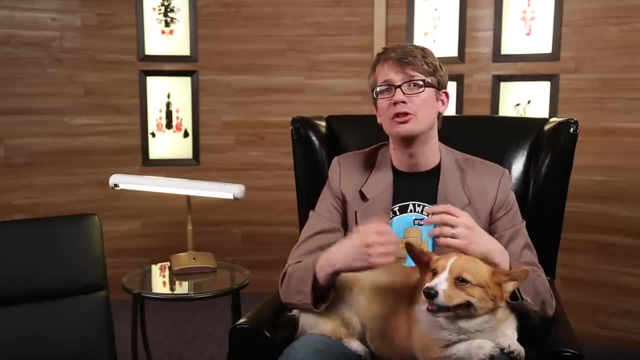 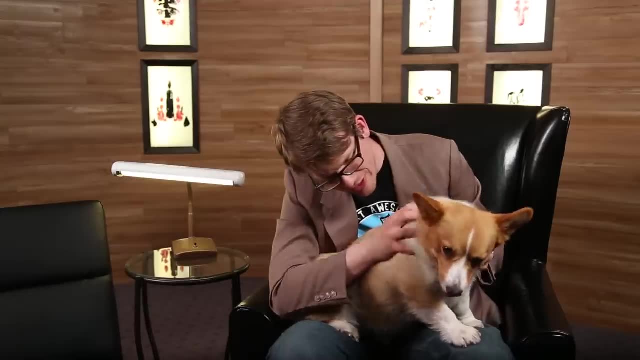 And yeah, I can tell with my eyeballs that some stars are brighter than others, but other stars They just look exactly the same to me. I can't tell the difference in their brightness. Are you done? Is it time for you to go? 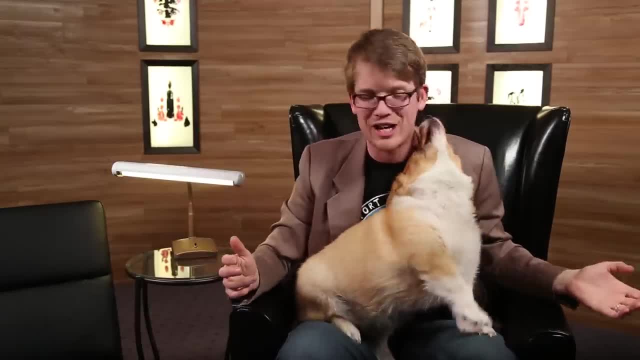 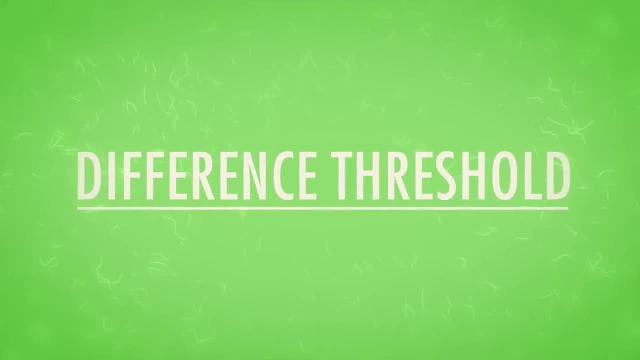 Gimme, gimme a Yes, yes, Okay, Good girl. The point at which one can tell the difference is the different threshold, But it's not linear, Like if a tiny star is just a tiny bit brighter than another tiny star. I can tell. 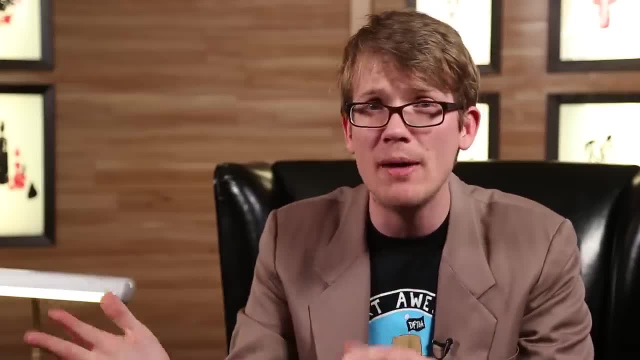 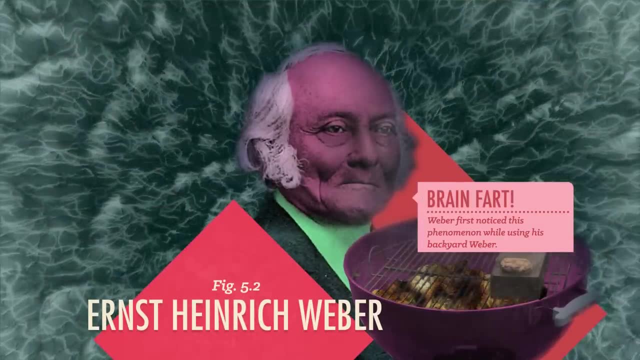 But if a big star is that same tiny amount brighter than another big star, I won't be able to tell the difference. This is important enough that we gave the guy who discovered it a law. Weber's law says that we perceive differences on a logarithmic, not linear, scale. 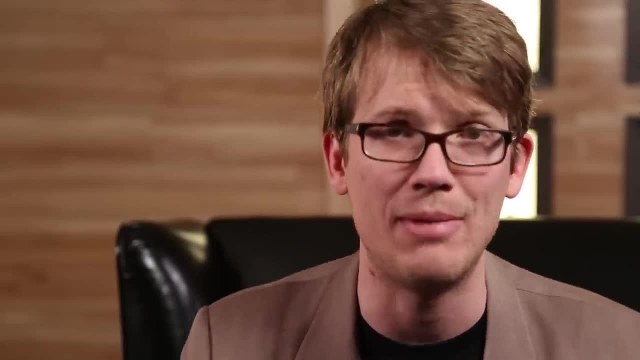 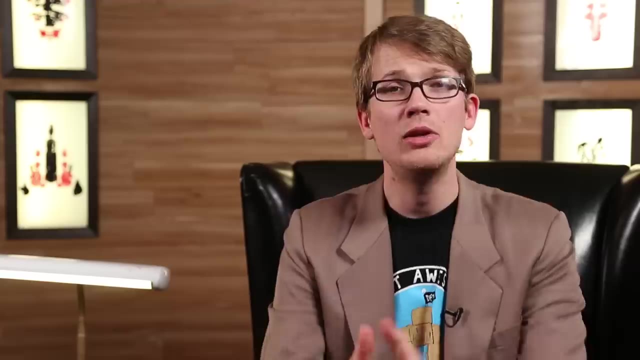 It's not the amount of change, it's the percentage change that matters. Alright, how about now? we take a more in-depth look at how one of our most powerful senses works: Vision. Your ability to see your face in the mirror is the result of a long but lightning-quick sequence of events. 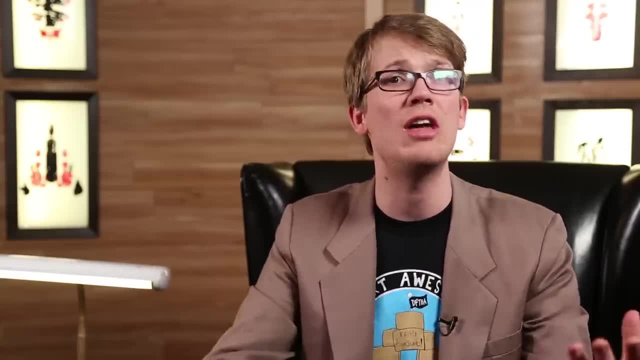 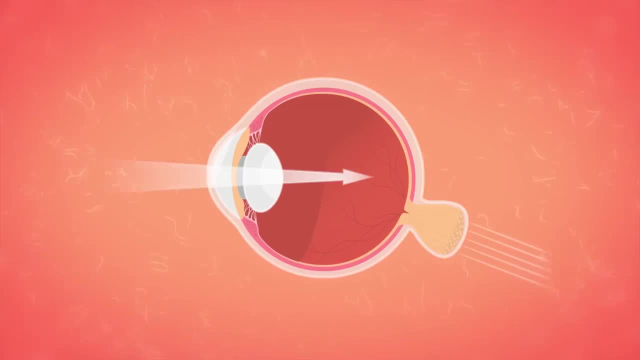 Light bounces off your face and then off the mirror and then into your eyes, which take in all that varied energy and transforms it into neural messages that your brain processes and organizes into what you actually see, which is your face. Or if you're looking elsewhere, maybe you see a coffee cup or a corgi or a scary clown. 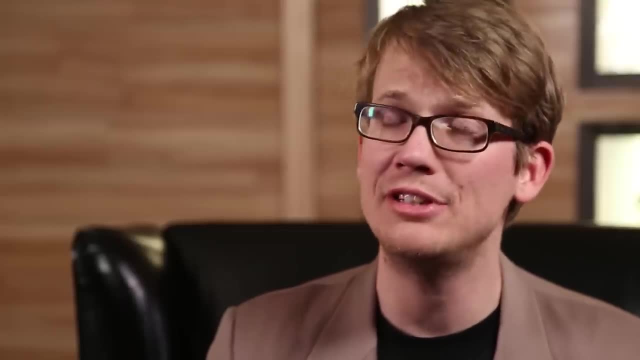 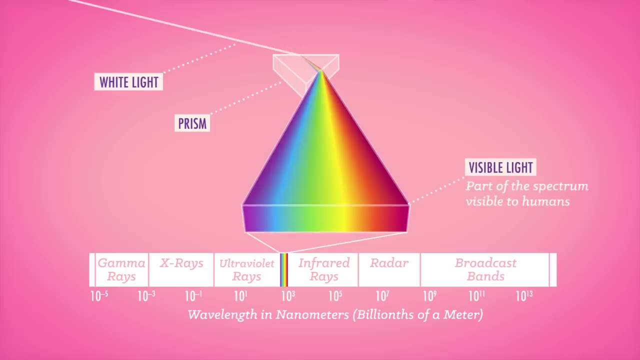 holding a tiny green pie. So how do we transform light waves into meaningful information? Well, let's start with the light itself. What we humans see as light is only a small fraction of the full spectrum of electromagnetic radiation that ranges from gamma to radio waves. 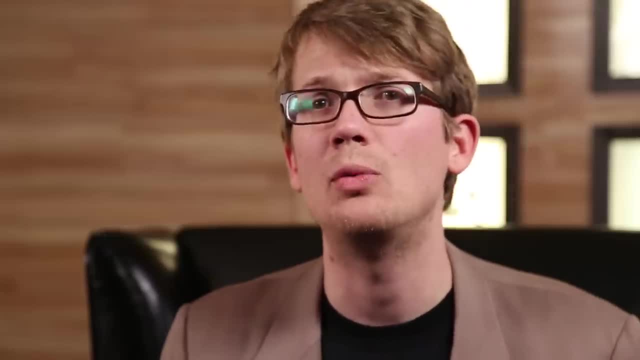 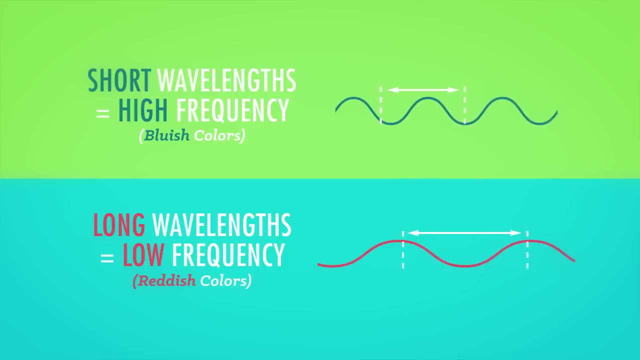 Now, light has all kinds of fascinating characteristics that determine how we sense it. But for the purposes of this topic, we'll understand light as traveling in waves. The wave's wavelength and frequency determines their hue and their amplitude determines their intensity or brightness. 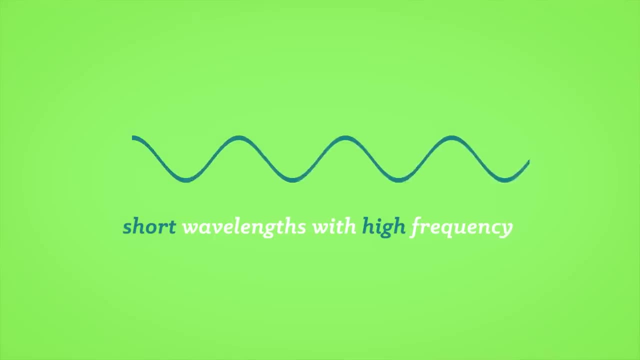 For instance, a short wave is light. It has a high frequency. Our eyes register short wavelengths with high frequencies as bluish colors, while we see long low-frequency wavelengths as reddish hues. The way we register the brightness of a color, the contrast between the orange of a Sherbert, 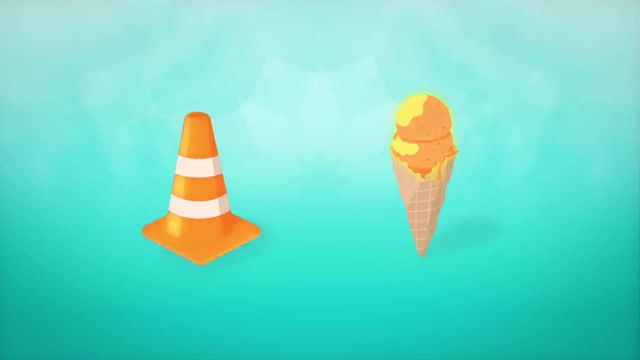 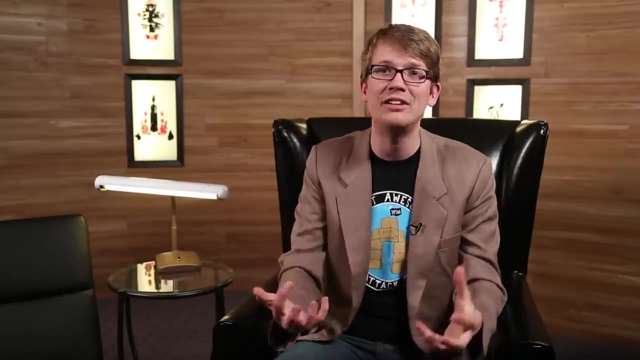 and the orange of a construction cone has to do with the intensity or amount of energy in a given light wave which, as we just said, is determined by its amplitude. Greater amplitude means higher intensity means brighter color. Someone just told me that Sherbert doesn't isn't a word that exists. 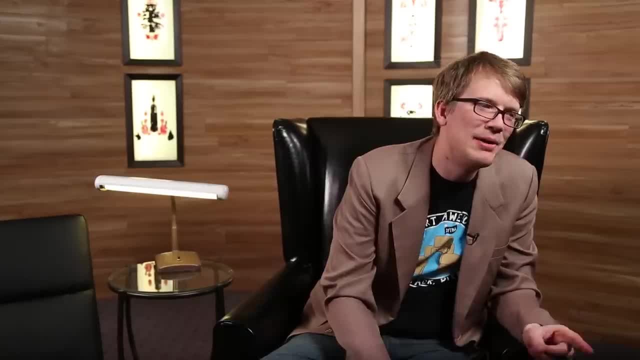 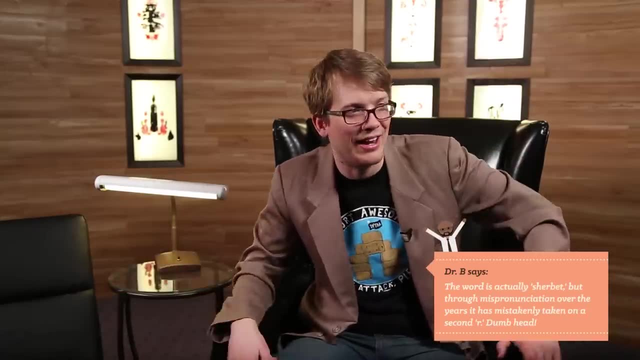 His name is Michael Aranda and he's a dumb head. Did you type it into the dictionary? Type it into Google? Ask Google about Sherbert. So Sherbert is a thing. So, after taking in this light through the cornea and the pupil, it hits the transparent disc behind the pupil, the lens. 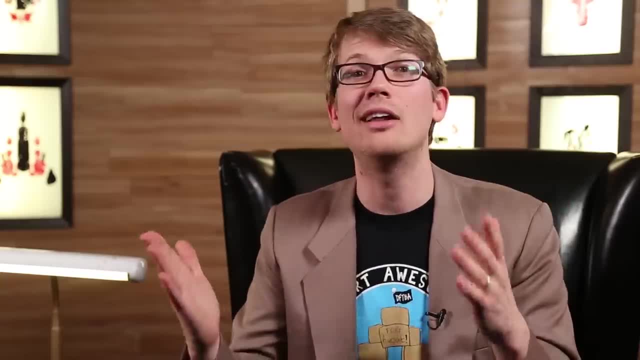 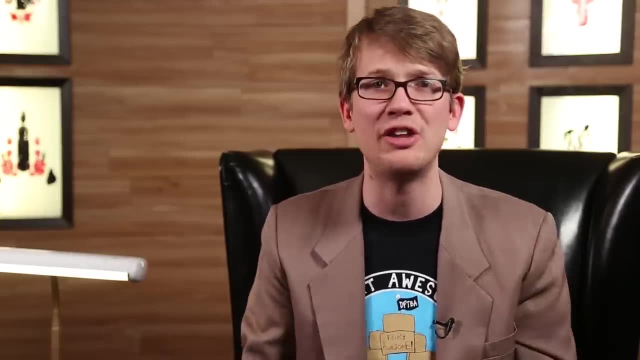 which focuses the light rays into specific images And, just as you'd expect a lens to do, it projects these images onto the retina, the inner surface of the eyeball that contains all the receptor cells that begin sensing that visual information. Now your retinas don't receive a full image, like a movie being projected onto a screen. 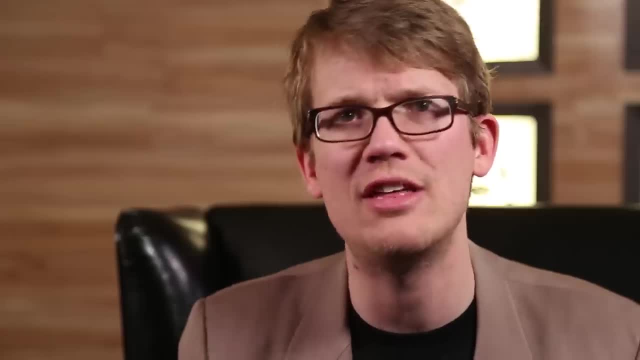 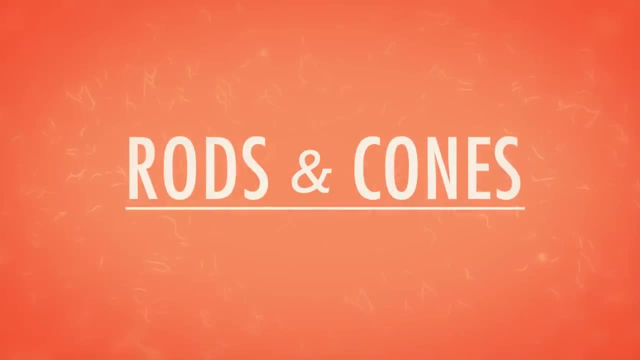 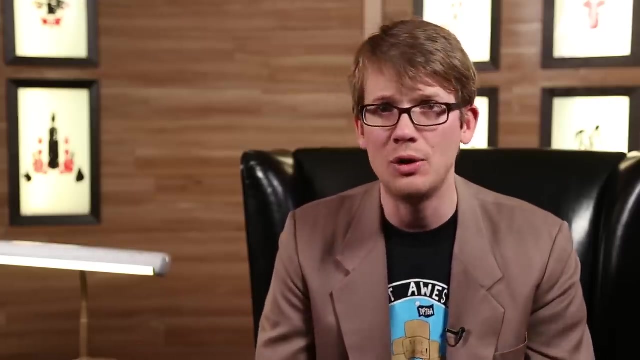 It's more like a bunch of pixel points of light energy that millions of receptors translate into neural impulses and zip back into the brain. These retinal receptors are called rods and cones. Our rods detect grayscale and are used in our peripheral vision as well as to avoid stubbing our toes in twilight conditions when we can't really see in color. 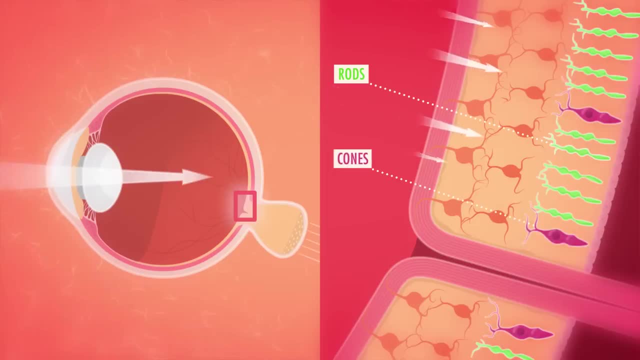 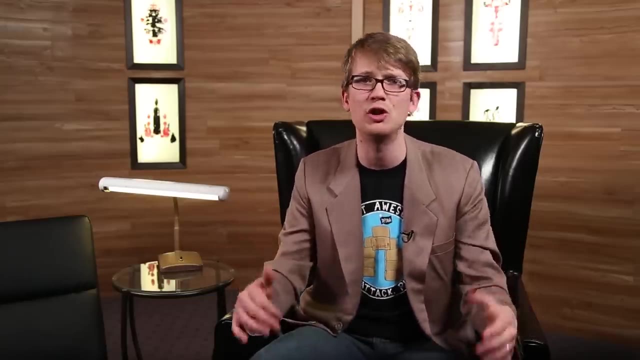 Our cones detect fine detail and color, Concentrated near the retina's central focal point called the fovea. cones function only in well-lit conditions, Allowing you to appreciate the intricacies of your grandma's china pattern or your uncle's sleeve tattoo. 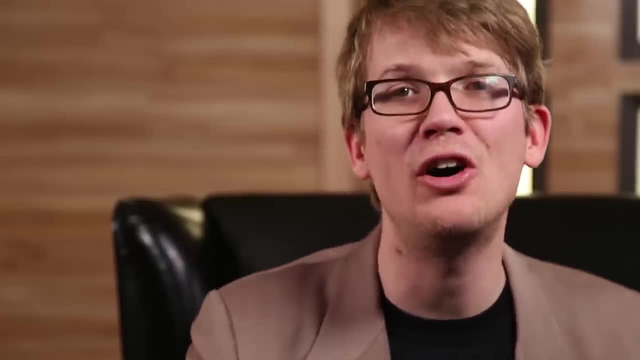 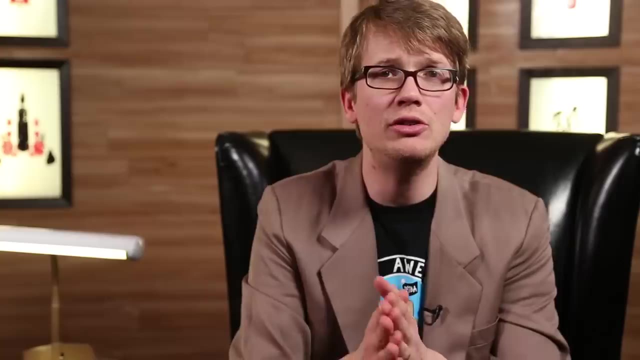 And the human eye is terrific at seeing color. Our difference threshold for colors is so exceptional that the average person can distinguish a million different hues. There's a good deal of ongoing research around exactly how our color vision works, but two theories help explain some of what we know. 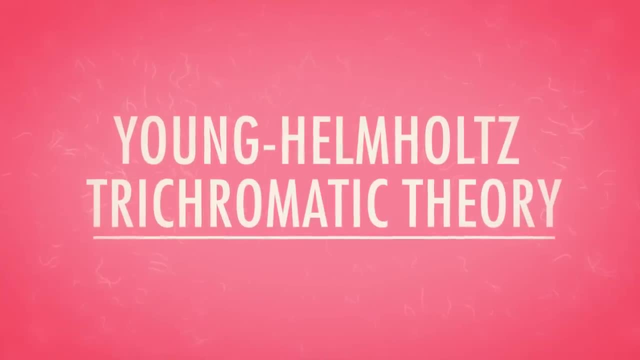 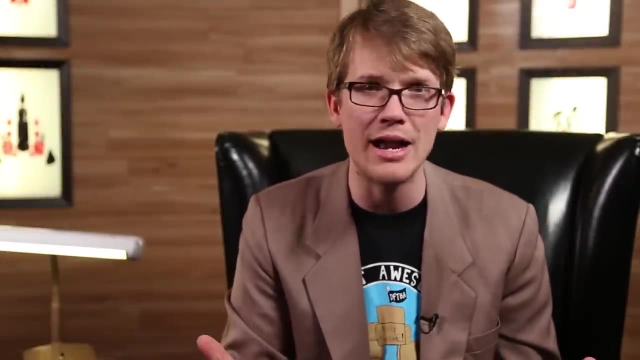 One model called the Young-Hemholtz trichromatic theory suggests that the retina houses three specific color receptor cones that register red, green and blue And, when stimulated together, their combined power allows the eye to register any color. 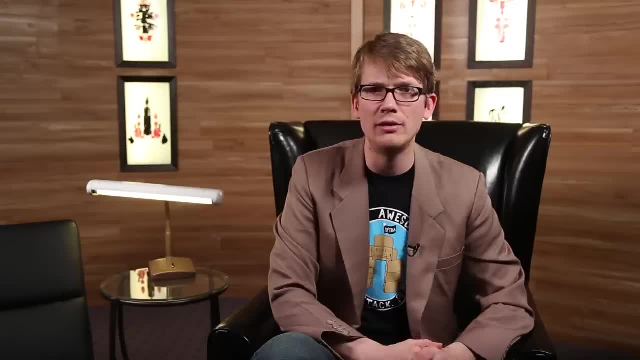 Unless, of course, you're color blind. About 1 in 50 people have some level of color vision deficiency. They're mostly dudes, because the genetic defect is sex-linked. If you can't see the Crash Course logo, pop out at you in this figure. 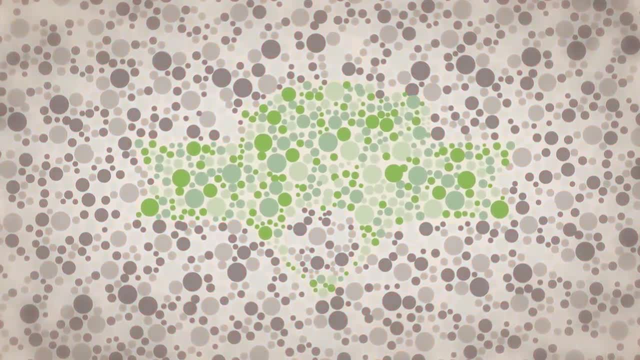 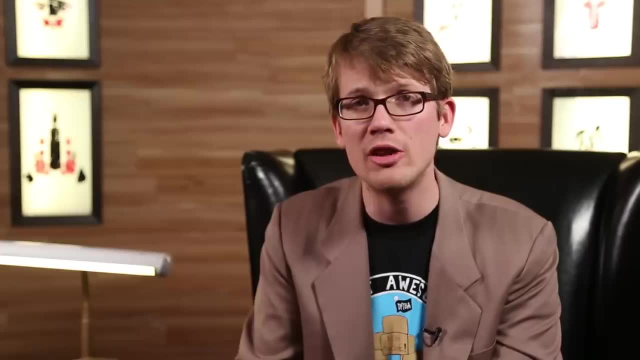 it's likely that your red or green cones are missing or malfunctioning, which means that you have dichromatic instead of trichromatic vision and can't distinguish between shades of red and green. The other model for color vision, known as the opponent process theory, 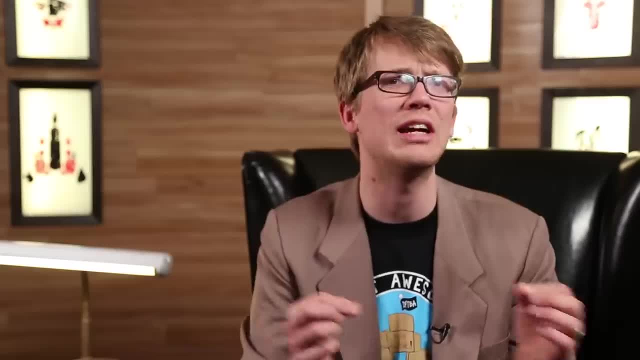 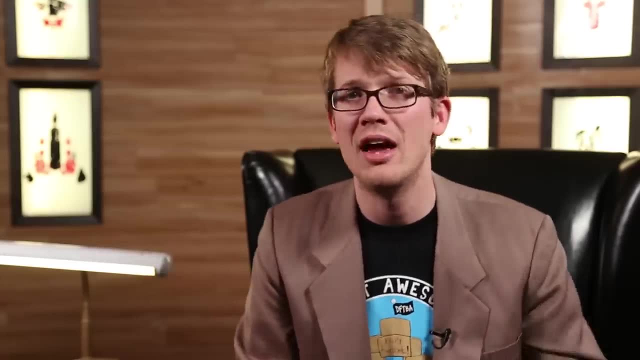 suggests that we see color through processes that actually work against each other. So some receptor cells might be stimulated by red but inhibited by green, while others do the opposite, and those combinations allow us to register colors. But back to your eyeballs. 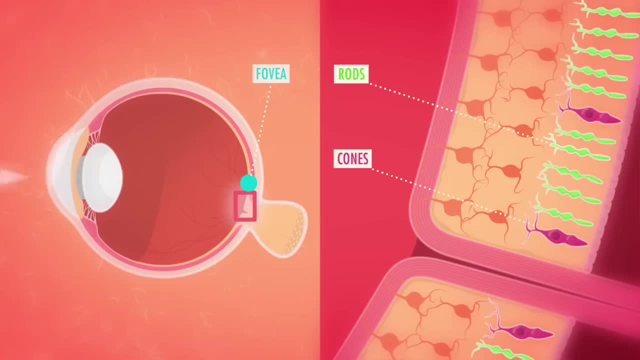 When stimulated, the rods and cones trigger chemical changes that spark neural signals, which in turn activate the cells behind them, called bipolar cells, whose job it is to turn on the neighboring ganglion cells. The long axon tails of these ganglions braid together to form the ropey optic nerve. 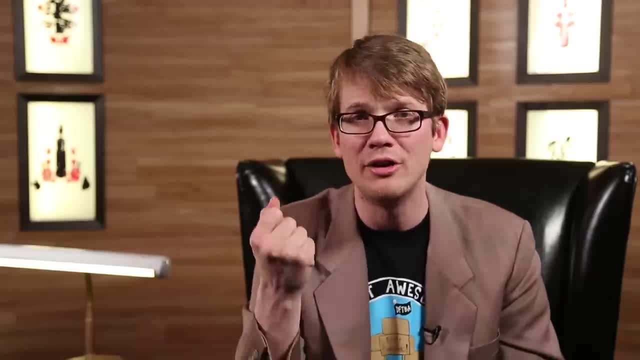 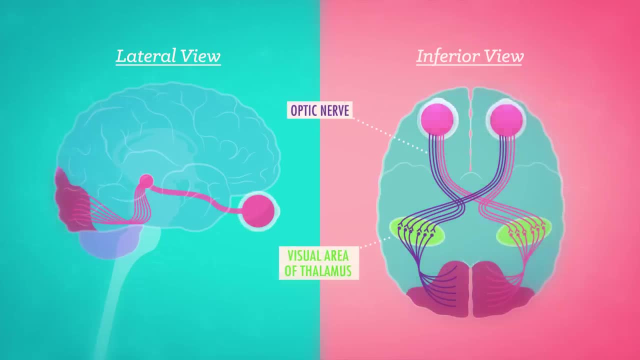 which is what carries the neural impulses from the eyeball to the brain. That visual information then slips through a chain of progressively complex levels as it travels from optic nerve to the thalamus and onto the brain's visual cortex. The visual cortex sits at the back of the brain, in the occipital lobe. 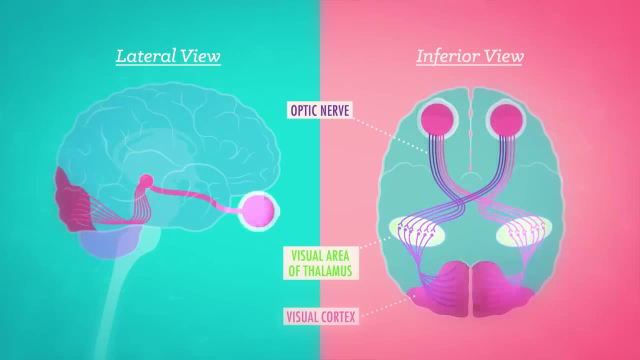 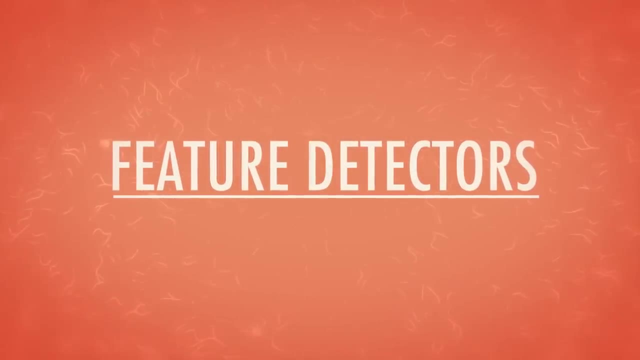 where the right cortex processes input from the left eye and vice versa. This cortex has specialized nerve cells called feature detectors that respond to specific features like shapes, angles and movements. In other words, different parts of your visual cortex are responsible for identifying different aspects of things. 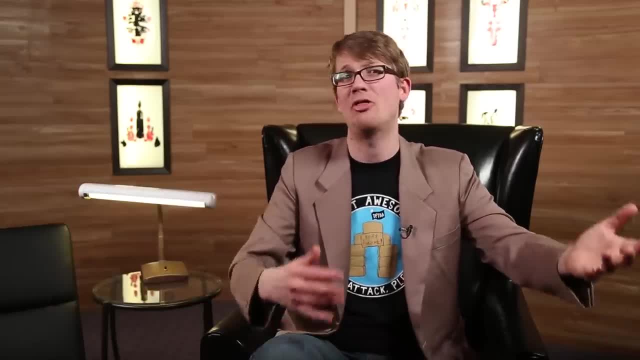 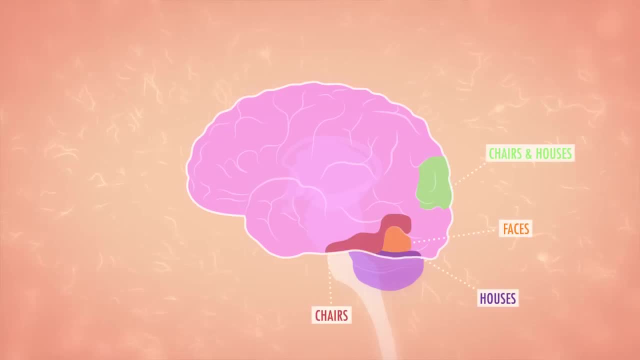 A person who can't recognize human faces may have no trouble picking out their set of keys from a pile on the counter. That's because the brain's object perception occurs in a different place from its face perception. In the case of Dr Sachs, his condition affects the region of the brain called the fusiform gyrus. 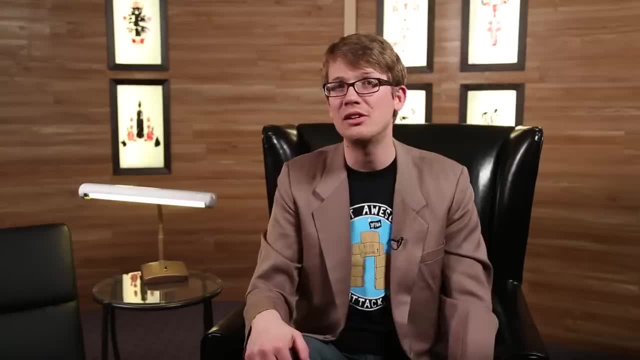 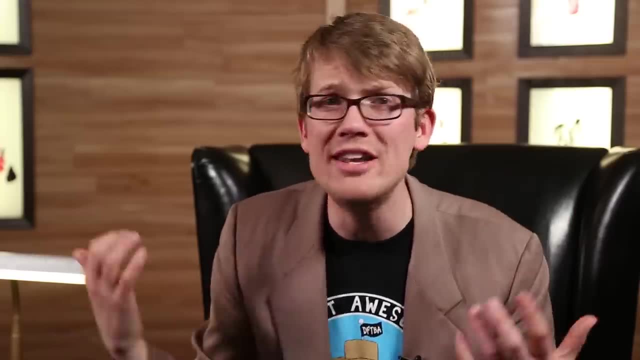 which activates in response to seeing faces. Sachs' face blindness is congenital, but it may also be acquired through disease or injury to that same region of the brain And some cells in a region may respond to just one type of stimulus, like posture or movement or facial expression. 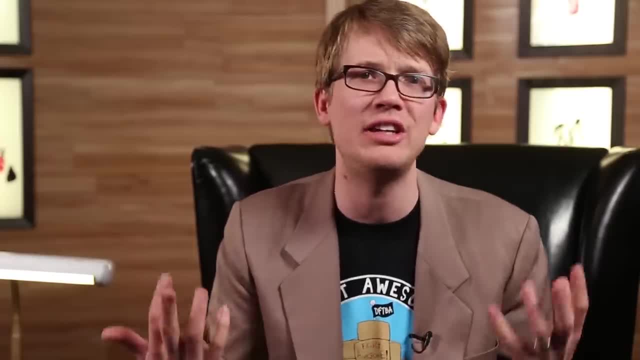 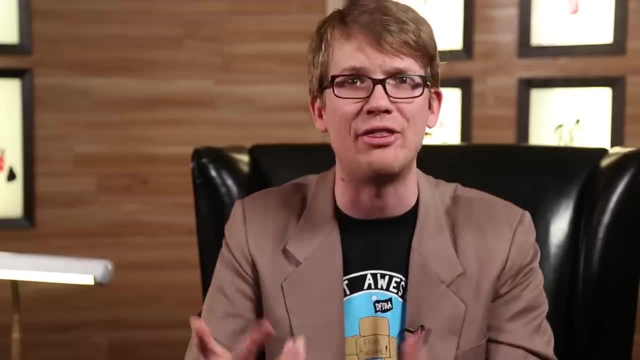 while other clusters of cells weave all that separate information together in an instant analysis of a situation. That clown is frowning and running at me with a tiny cream pie. I'm putting these factors together. Maybe I should get out of here. This ability to process and analyze many separate aspects of a situation at once is called parallel processing. 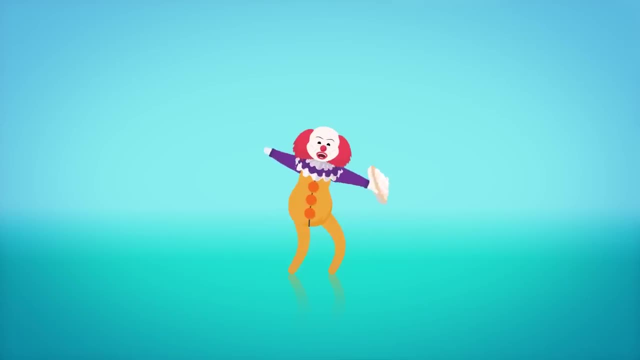 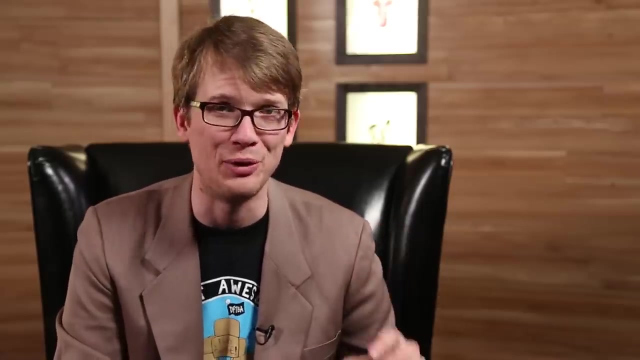 In the case of visual processing, this means that the brain simultaneously works on making sense of form, depth, motion and color, And this is where we enter the whole world of parallel processing. It's called perception, which gets complicated quickly and can even get downright philosophical. 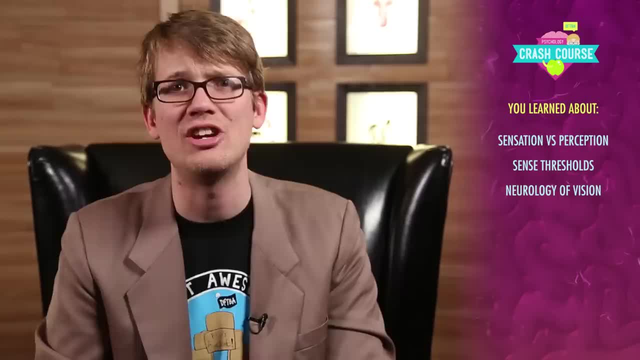 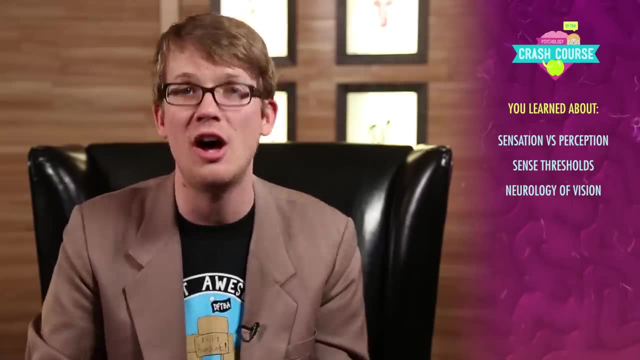 So we'll be exploring that in depth next time, but for now, if you were paying attention, you'll learn the difference between sensation and perception, the different thresholds that limit our senses and some of the neurology and biology and psychology of human vision. 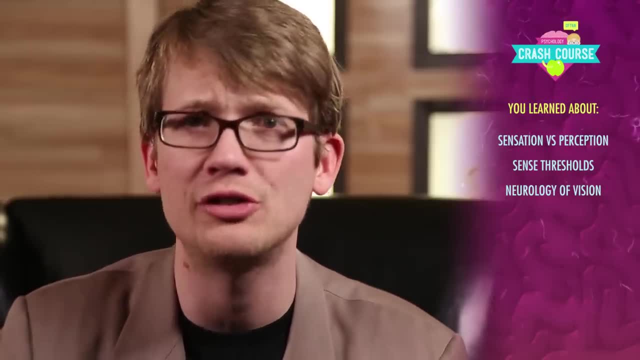 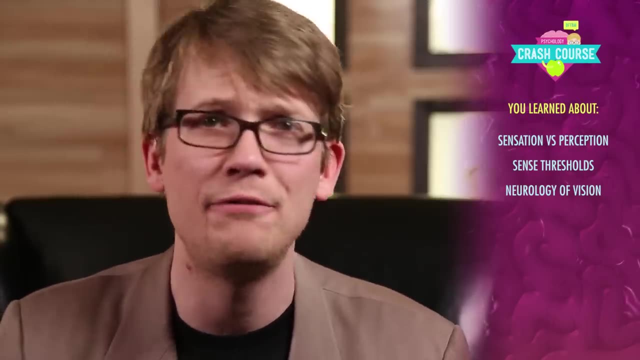 Thanks for watching this lesson with your eyeballs and thanks to our generous co-sponsors who made this episode possible: Alberto Costa, Alpna Agrawal, PhD, Frank Zegler, Philip Detmer and Kurtzgesagt. 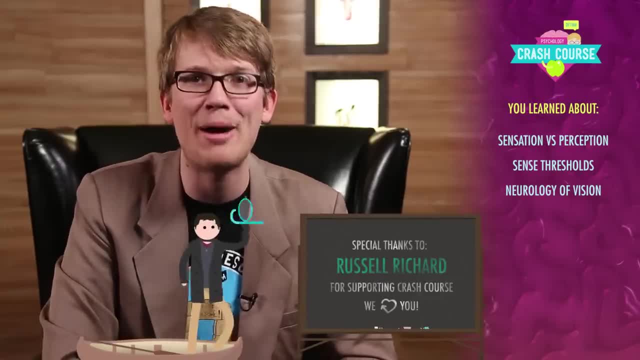 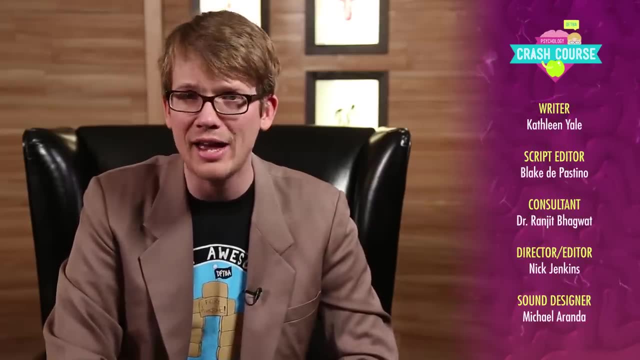 And if you'd like to sponsor an episode and get your own shout-out, you can learn about that and other perks available to our Subbable subscribers. Just go to subbablecom slash crashcourse. This episode was written by Kathleen Yale, edited by Blake DePastino. 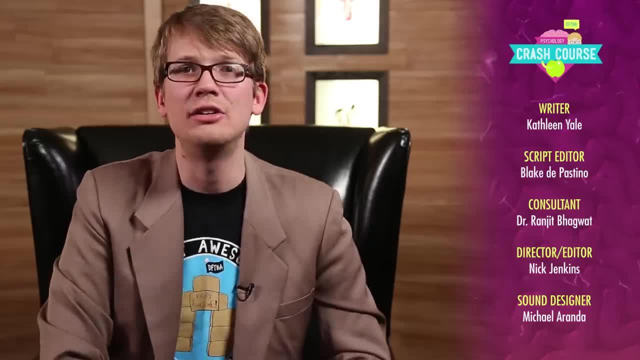 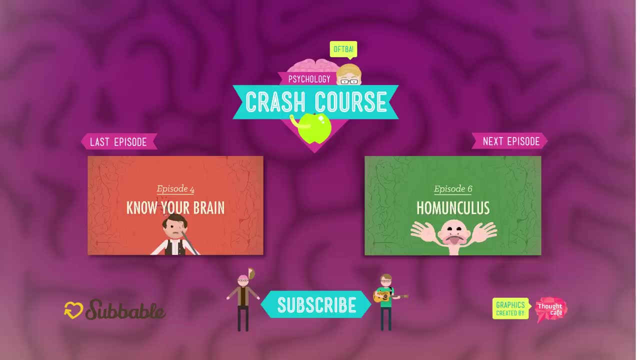 and our consultant is Dr Ranjit Bhagwat, Our director and editor is Nicholas Jenkins, The script supervisor is Michael Aranda, who is also our sound designer, and our graphics team is Thought Cafe. Thank you for watching.